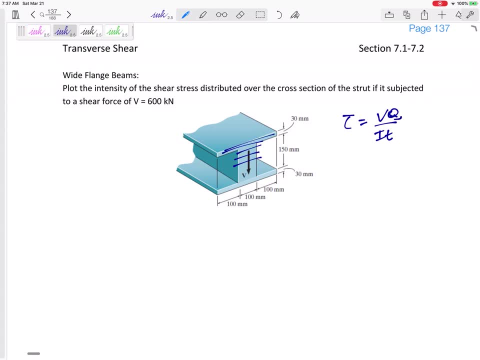 different locations. right, the Q and the T are different. So what I want to do is I want to plot. I'll look at a few important locations, like maybe the very top- Let's see what it's doing- kind of right above, right below, where this top flange starts, and maybe at the middle, I think. 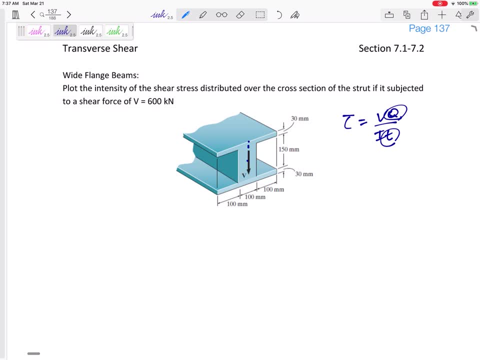 that'll be enough to to plot the intensity of the shear stress. So before I get too far, let me find the I. So for this shape, I think it's easiest to do 1 twelfth of the whole rectangle and minus these two. 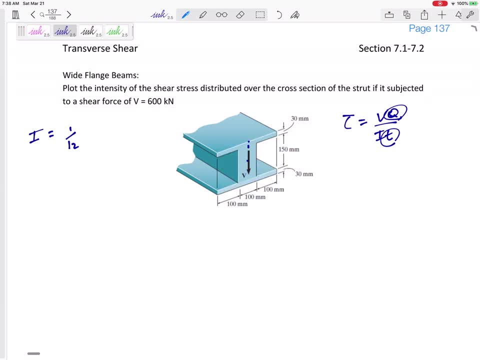 rectangles right here. So 1 twelfth, let's see 300 height, 210 cubed minus 1 twelfth of 100 uba, OK, of 150 cubed, and there are two of those. so I've got the eye of 1.75 times 10 to. 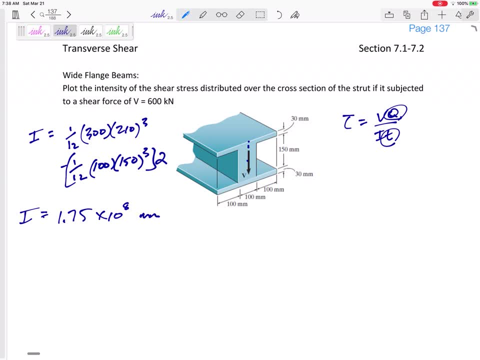 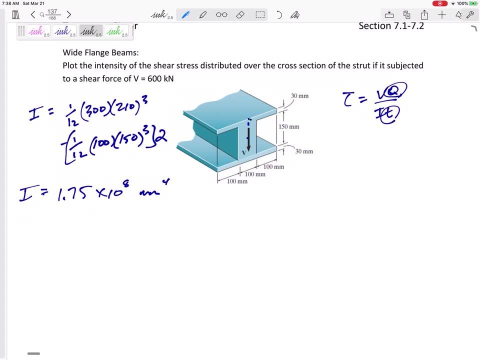 the 8, and everything was in millimeters, that's in millimeters to the fourth. all right, so that's the eye for the whole shape. that's the eye, no matter whether I'm looking at the very top, middle, bottom, wherever. all right, so let's look. 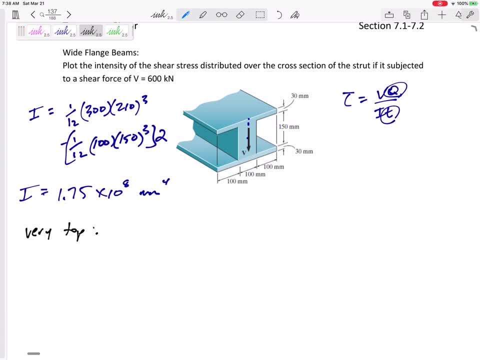 at the very top tau VQ over IT. remember, at the very, very top of the very bottom, at zero, and mathematically that's true, because inside of this Q, Q is y, bar prime, a prime, the a prime is the area past your point, area away from the. 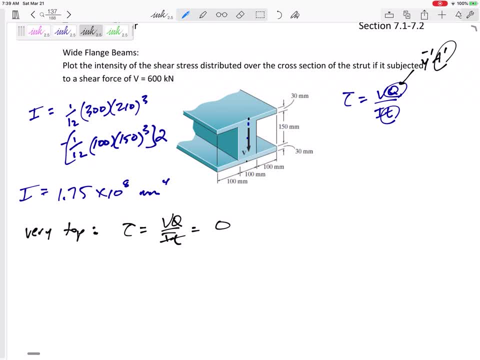 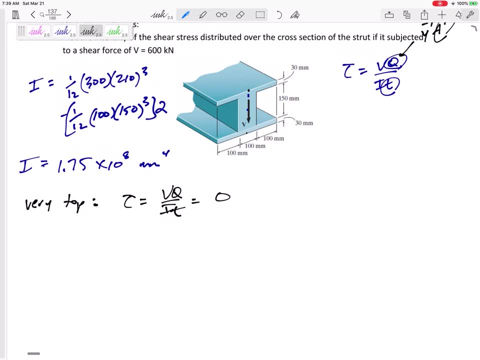 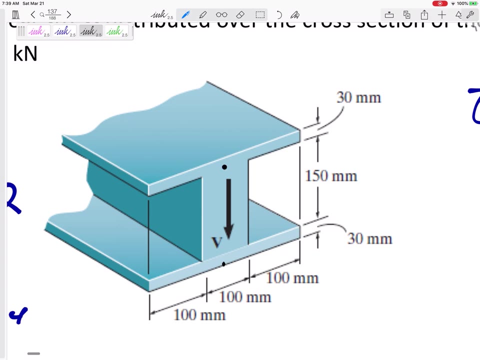 neutral axis you, and that that would be zero. so the shear stress at the very top would be zero. alright, so how about we look now at? it's going to kind of change right here where this top piece changes. so I'm going to look at both right above. 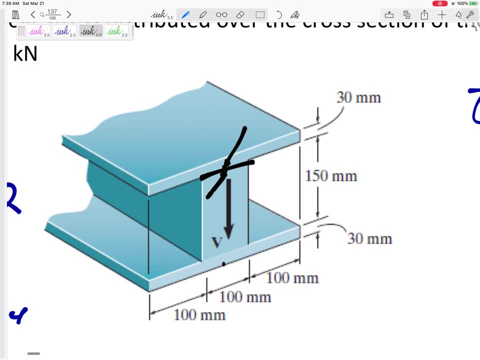 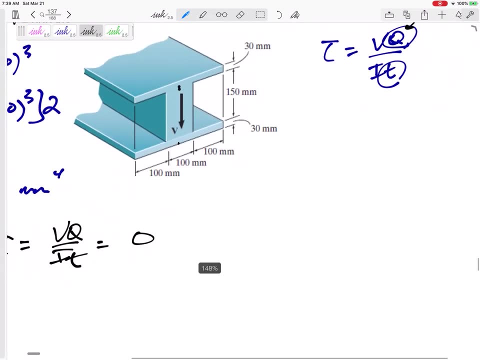 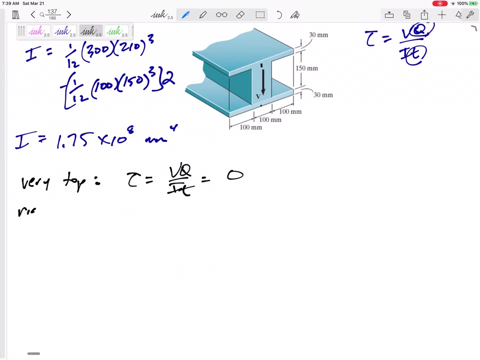 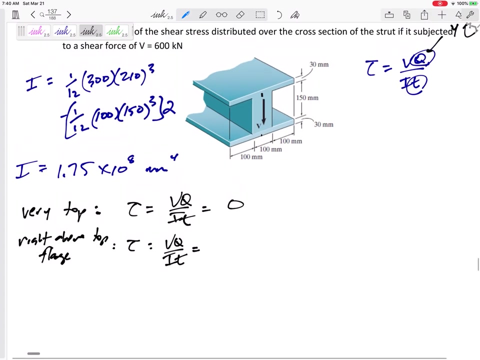 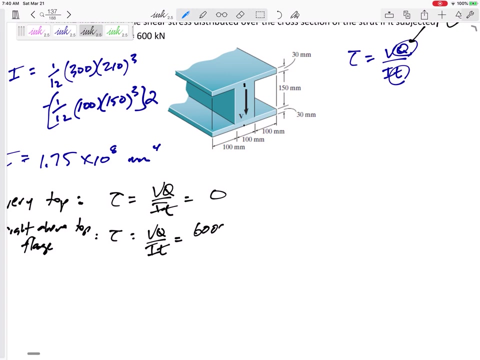 to where this lets call And right below where this top part meets, right here. so let's do right above. so this would be right above top flange. All right, the V: 600 kilonewtons, I'm going to do 600,000 newtons. 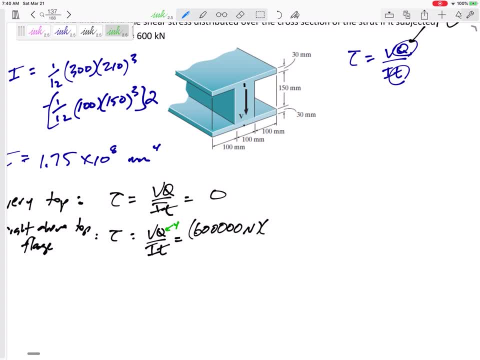 The Q. All right, so Q is Y bar prime, A prime. Y bar prime. I'm going to come back to The A prime would be the area away from this. So this would be a 30 by 300.. So this would be 300 by 30.. 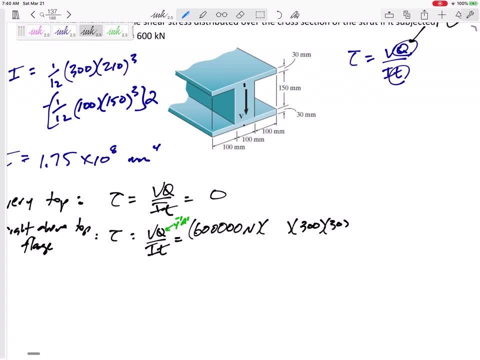 All those are millimeters. And now the Y bar prime is not the distance to the point. The distance to the point would just be 75.. But I need to go to the centroid of the A prime, So I would go 75.. 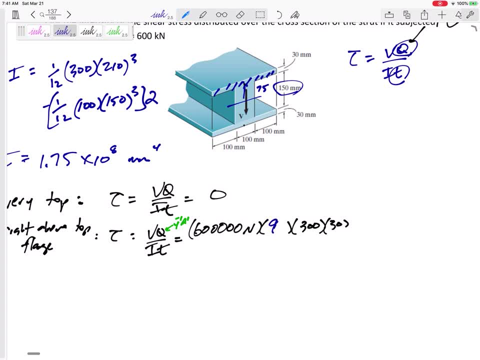 Plus 75.. Plus another 15. So my Y bar prime would be 90.. Got that All right. then the I, 1.75 times 10 to the 8, millimeters to the 4th, All this is millimeters, millimeters, millimeters, newtons. 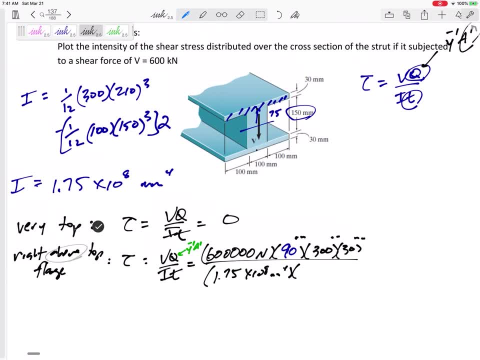 And then the thickness. All right, so above right here, the thickness would be 300.. All right above right here, Thickness would be 300.. So this would be 9.24 megapascals, 9.24 MPa. 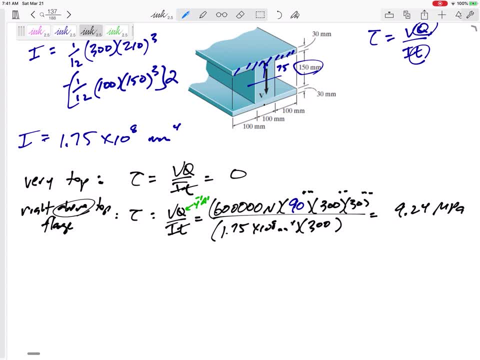 Now I'm not going to say positive or negative. If the V is down, then all of this shear stress is down, Everywhere it's down. It's down here, here, here It's down. Okay, so let's do right below. 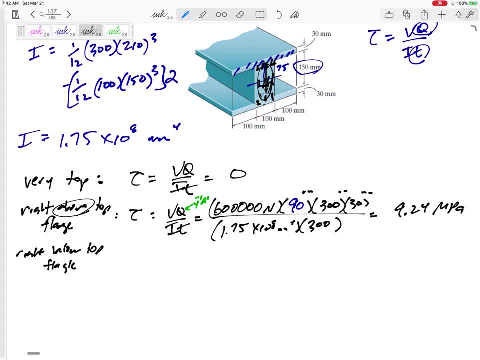 So that point: VQ over IT. Let's think about this. Everything stays the same: 600,000, 90,, 330.. I'm basically at the same point. So I'm not changing the Y prime or A prime. 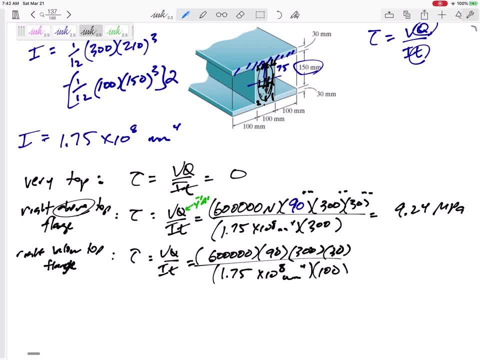 But here I am changing the thickness T. I am changing thickness T. How does that change this? The shear stress would be 27.7 MPa. So it's like this immediate jump of thicknesses and so an immediate jump of shear stress. 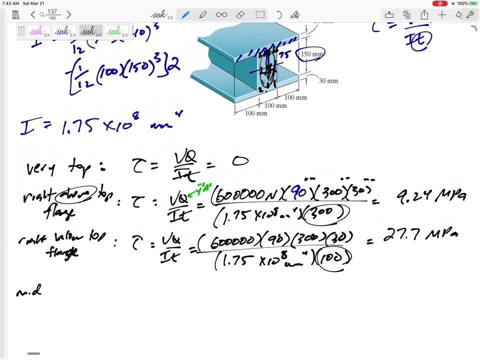 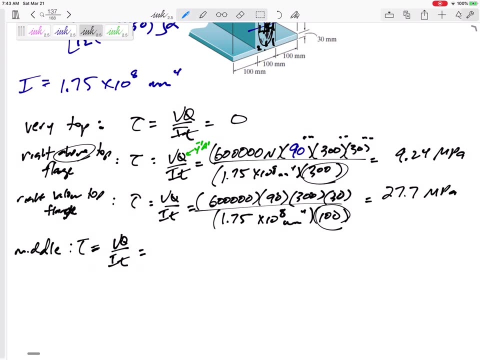 All right, then let's look at the middle. All right, the middle. let me see if I have room for this would be V: 600,000 newtons. Q- All right, so this one, if we're looking at the middle. 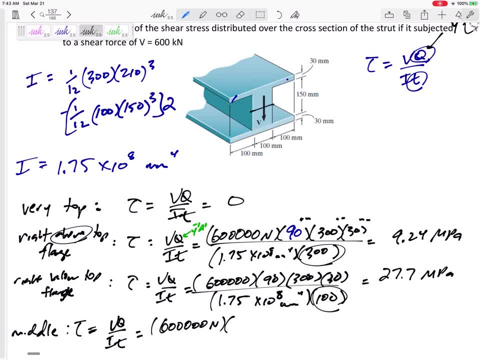 I think it makes most sense to do the Q. We talked about this, We talked about the T here. So if I want to find the Y bar, I can just break it up into Y bar prime, A prime of that A prime and that A prime. 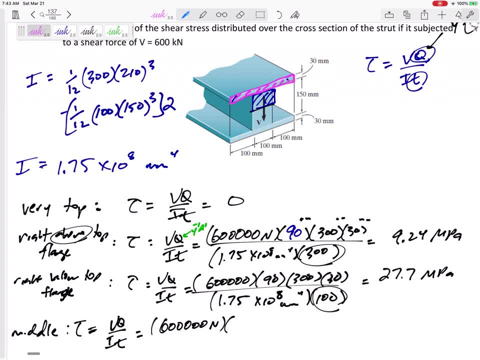 The A prime above the middle part would look like a T. So if I don't want to find the centroid of that T- because Y bar prime is from the neutral axis to the centroid of A prime, if I don't want to do a centroid of a T, 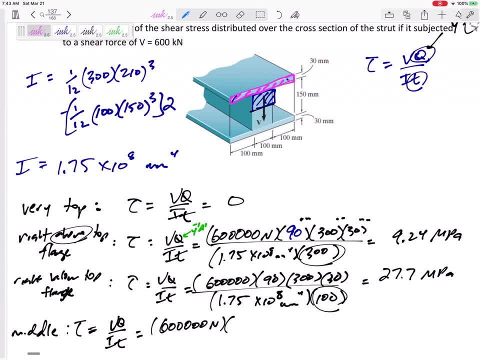 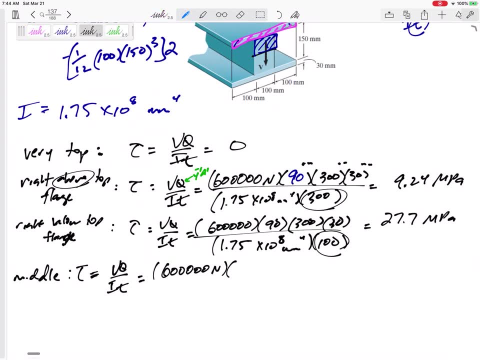 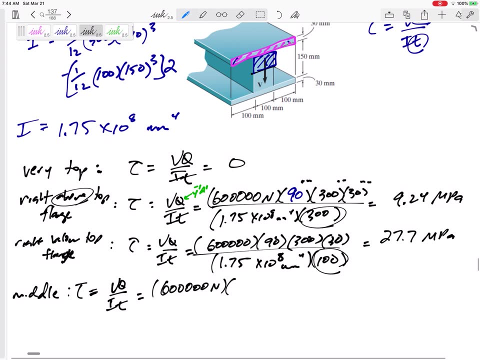 I can just break it up into Y bar prime, A prime of the blue rectangle, plus Y bar prime, A prime of the blue rectangle, prime of the pink rectangle. So that's what I'm going to do: Y bar prime, A prime of the. 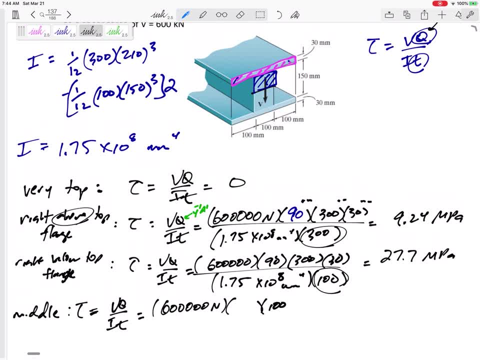 blue. So let me do the A prime of the blue. It's 100 by 75.. And then the Y bar prime would be: from the neutral axis to the centroid of that would be 37.5.. And then the pink. I kind. 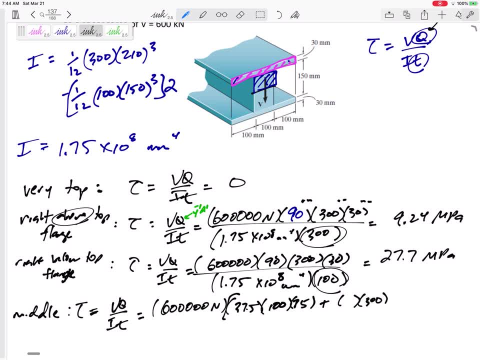 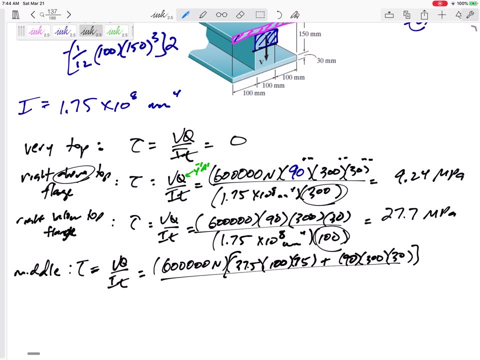 of already did that, The area would be 300 by 30 and the Y bar prime would be 90 to get to the centroid of that A prime. So just add those Y bar prime A primes up. That would be the cube at the middle. 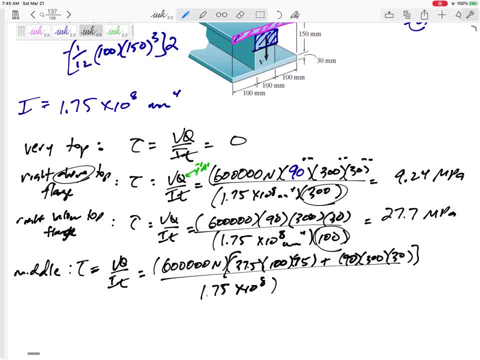 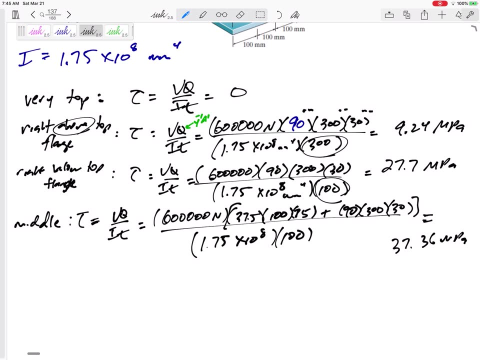 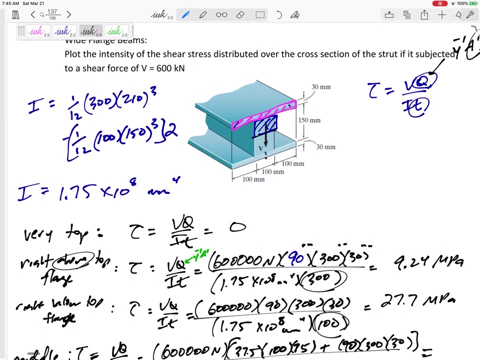 The I: 1.75 times 10 to the 8.. The thickness of the middle: 100.. So this would be 37.36 MPa. 37.36 MPa. Now, if I kept on doing this, because the shape is symmetric, the tau would. 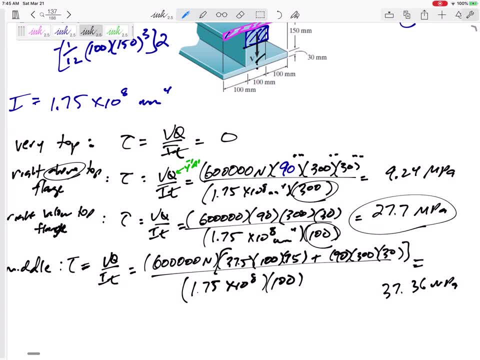 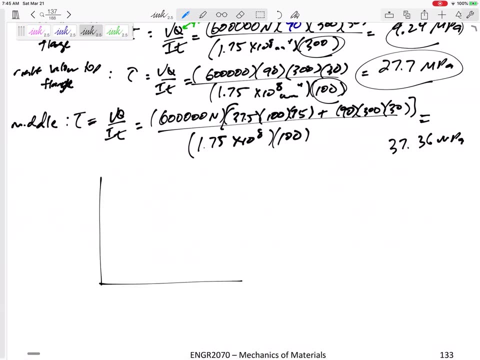 be symmetric, I would get 27.5.. 27.7 down here, 9.24 down there and 0,, of course, down there. All right, so let's kind of plot what this looks like over that shape. So let's look at the very top, very bottom. 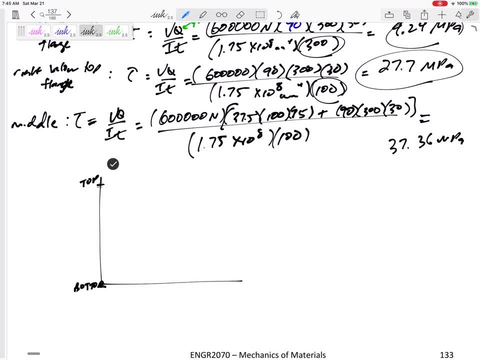 It starts at 0, ends at 0.. Now, if this was a solid rectangle, this would look like a parabola Maximum right here, And so this Q right here has this kind of shape, But for us it does. 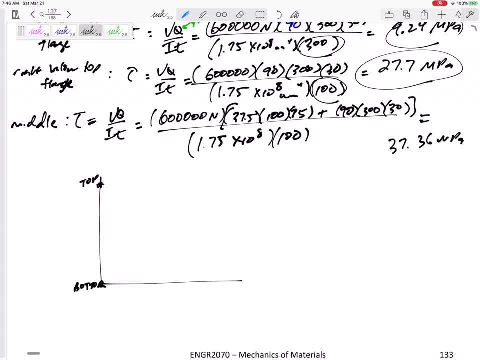 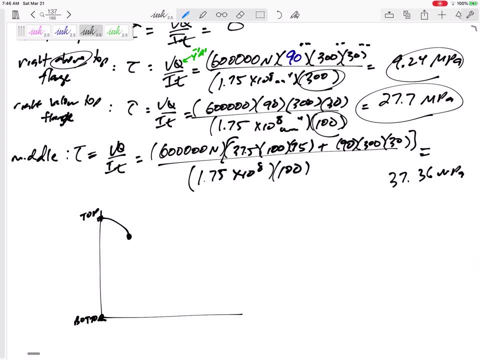 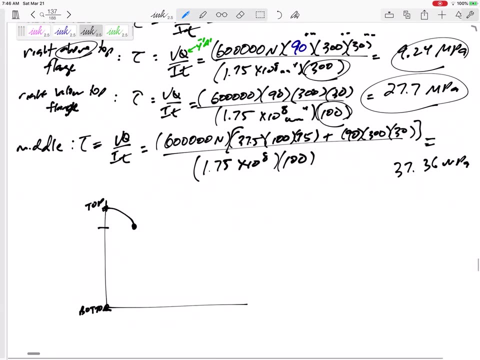 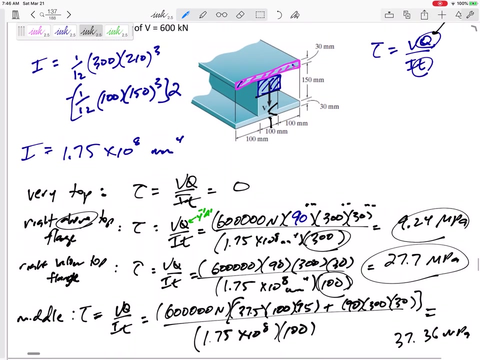 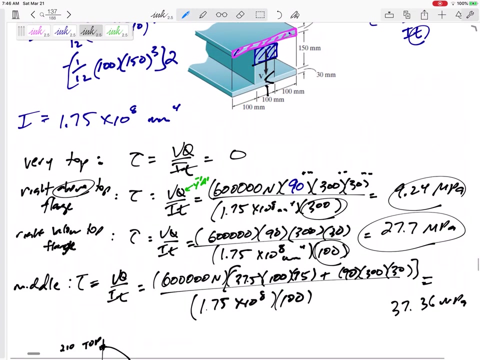 this shape. It doesn't really flatten out just yet. It does this shape until it gets to right here. So let's say this is, Let's say this is a 210 tall at let's see 180.. And this one would be 105, would be the. 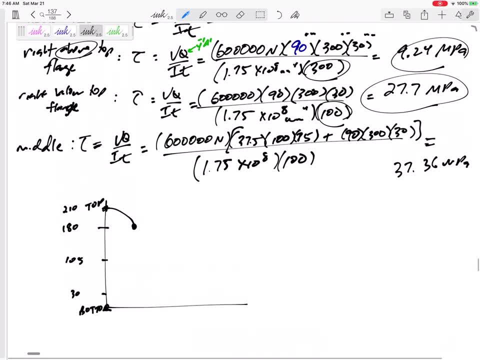 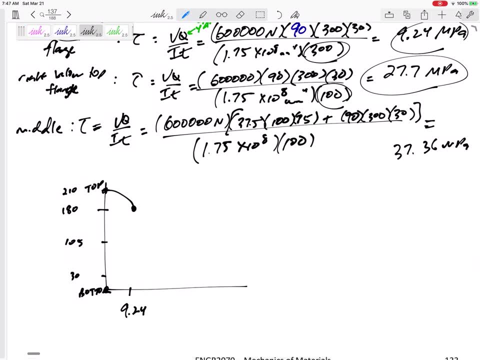 middle And this would be 30. So at this top flange it goes from 9.4 to 9.4 MPa. So this 9.4, so this, let's say this is the tau, This is the height h. It goes from 9.24 immediately.